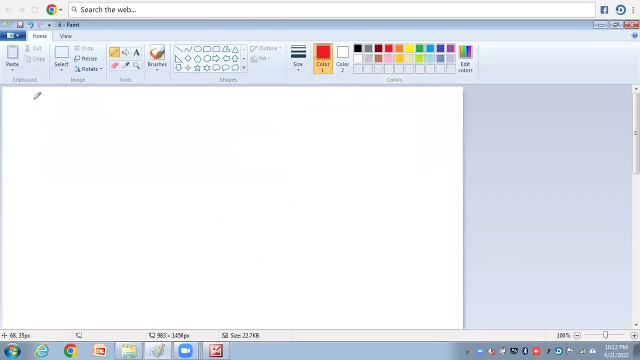 In this class. I would like to discuss about Gauss law, definition and derivation. It is also one of the Maxwell's equation- okay, Gauss law and R Maxwell's equation by A- Okay, This Gauss law constitutes one of the fundamental laws of electromagnetism. 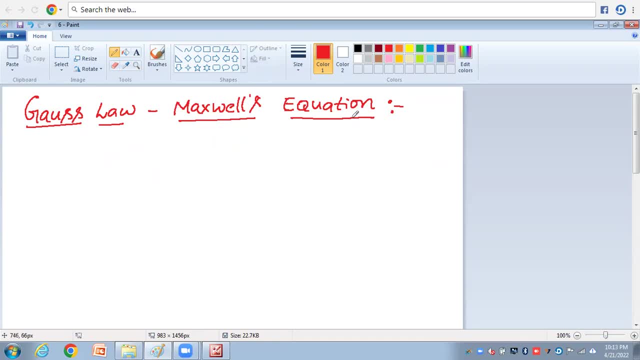 Okay, This Gauss law constitutes one of the fundamental law of electromagnetism. Let us start with this definition. Okay, About this Gauss law. Now. Gauss law states that the total electric flux- total electric flux denoted with the psi, total electric flux. While I am writing this, 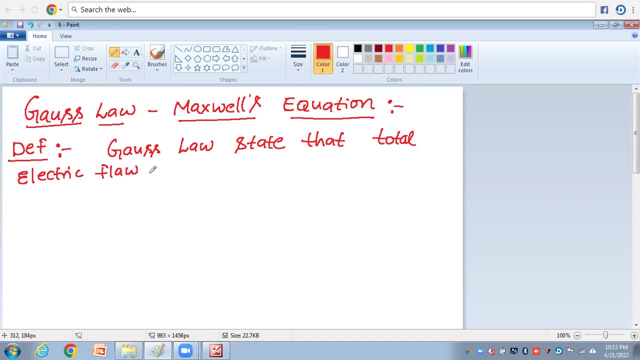 law. please try to remember this definition: Total electric flux denoted with psi through any closed surface. Okay, Through any closed surface. I will show that diagramed representation. Also, give me some time, After writing this equation, I will give some diagram awitical representation. 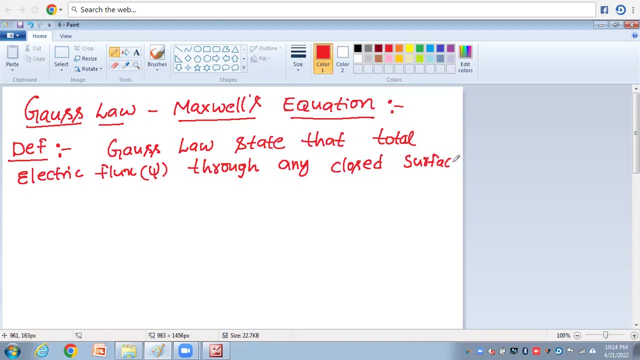 Also, closed surface is equal to the or same as the is equal to the total charge is equal to the total charge denoted with total electric flux. This shape is used so as to diffuse energy. This shape渐 missile will decrease. This shape is directly linked to both the. 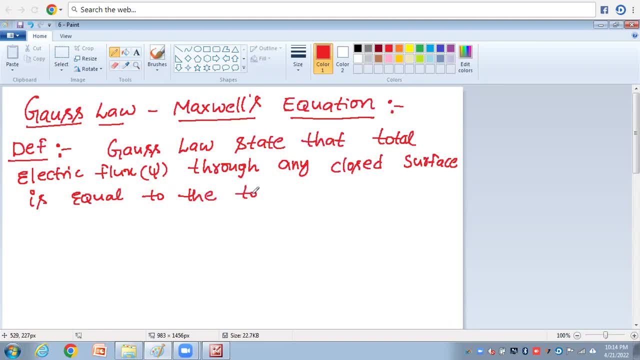 electrons. So as there are atoms in the electrical operation금, as there is a another꺼 open-out electrical energy in the electrical operation금, we can see that the close its appearencing also on this electrical environment. We are all washing. There are far off electrons in our production. The force is applied by voltage. The new premium can press ث scary one of these Rabot. it causes a small effect on the electrical system. узнается cz there. as a larger charge. I want to enjoy disrupted nie direction westarnos. 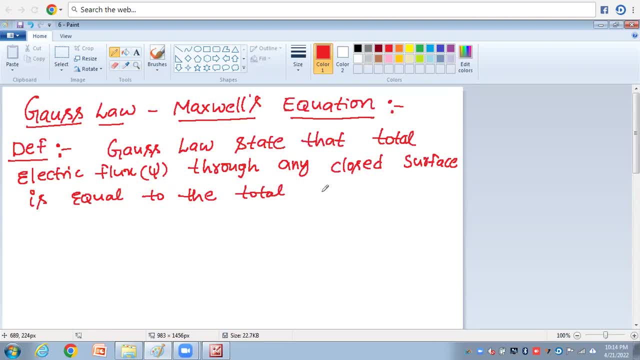 total charge denoted with n. total charge enclosed by that surface, enclosed by that same surface. okay, this is the definition of the Gauss law. right again, I will tell you. Gauss law states that's the total electric flux in any closed surface, any closed surface denoted with psi. there is a field component here, d bar. 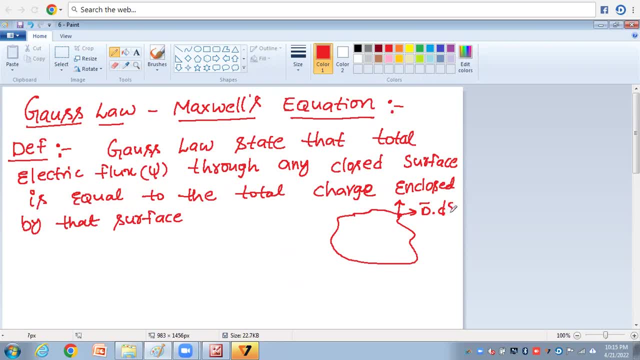 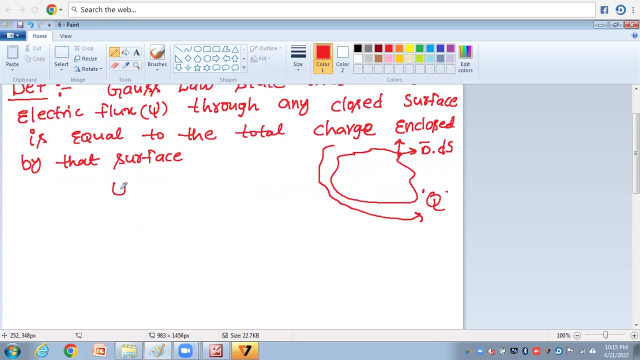 so any closed surface d bar dot ds is equal to the total electric flux total charge. total charge q and closer to that surface. okay, right now I will start with the definition. after this definition, I will start with the equation part. now, the total electric flux psi is equal to the total charge. 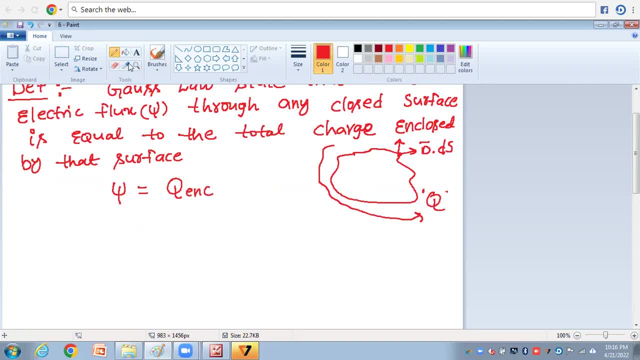 and closer to that surface. okay, based on this expression, I have written this mathematical form. okay, this ENC means enclosed. you have to write in the suffix of this q, right? this is the psi. electric flux is equal to the total charge enclosed in that surface. okay, now this psi is equal to the 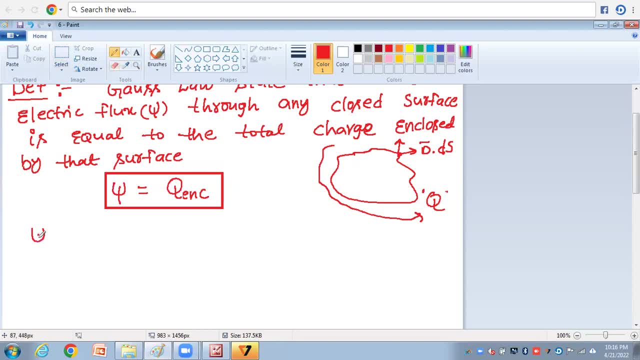 whole portion of t derived in electric flux density. okay, this is about psi equal to integral: d bar dot ds. okay, this is extended to psi equal to double integral. okay, when, if you write this surface or area, you go with the double integral, this is called d bar dot ds. right now coming to charge, 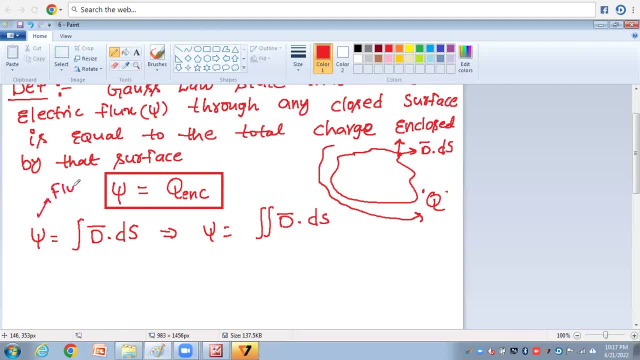 this is about flux. now i will discuss about the charge is denoted with q. okay, this is equal to the integral rho v total y volume charge: rho v- dv. okay, now i will take the boxes or i will write the expression names. this is equation one. this is equation two is substitute in equation a. we may do any type of. 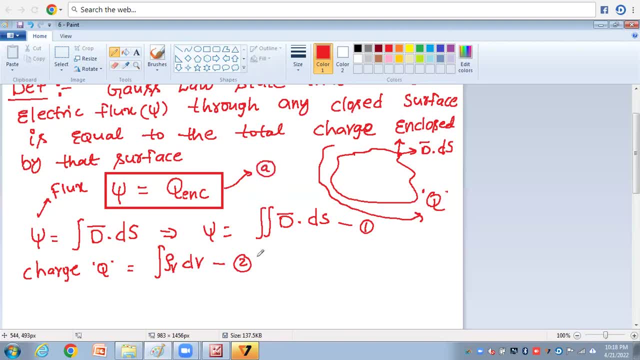 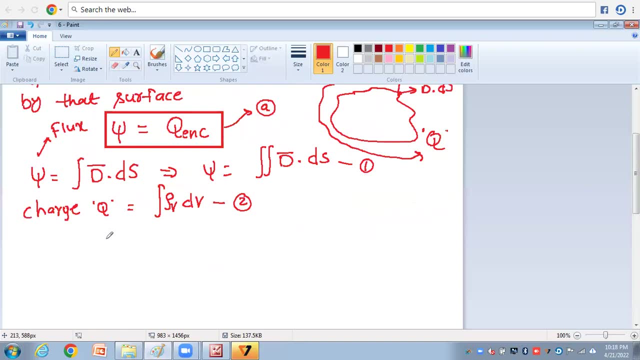 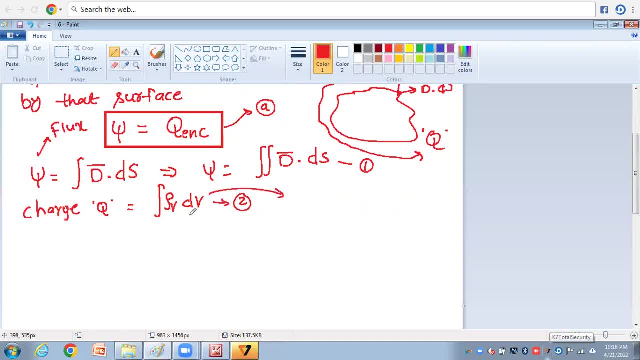 now psi equal to here. uh, i will extend a little bit. about this one. this is volume charge density about this one. this is volume charge density about this one. this is volume charge density. so this is v means volume. i will go with the. so this is v means volume. i will go with the. 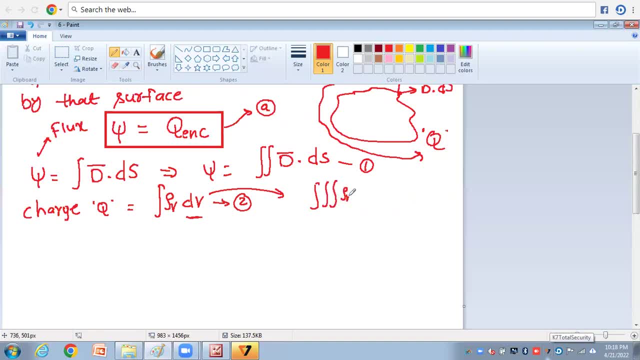 so this is v means volume. i will go with the triple integral. i will go with the triple triple integral. i will go with the triple triple integral. i will go with the triple integral, integral integral. rho v dv right. this is about the rho v dv right. this is about the. 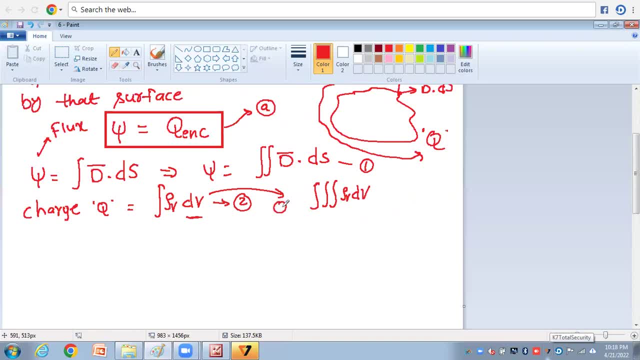 rho v dv. right, this is about the charge. okay, fine, this is about the charge. okay, fine, this is about the charge. okay, fine, this is about the charge. charge, charge, right, right, right, right right. this is very, very important discussion. this is very, very important discussion. this is very, very important discussion, while solving this expression once again. 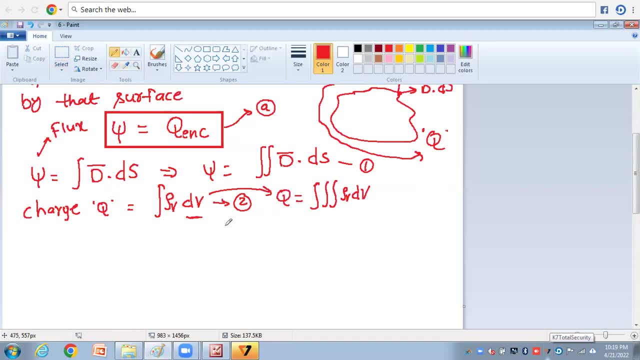 while solving this expression once again. while solving this expression once again, i will write about this one. this is, i will write about this one. this is, i will write about this one. this is about the charge, about the charge, about the charge. now, this one and the two expressions is. 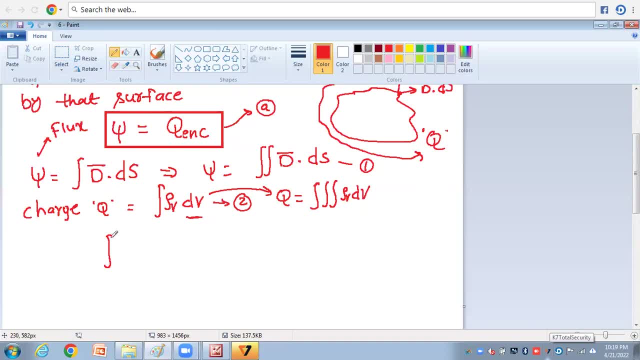 now this one and the two expressions is now this one and the two expressions is substitute in the equation, a substitute in the equation, a substitute in the equation a. then then, then i will write, i will write, i will write double integral, double integral, double integral d bar dot. 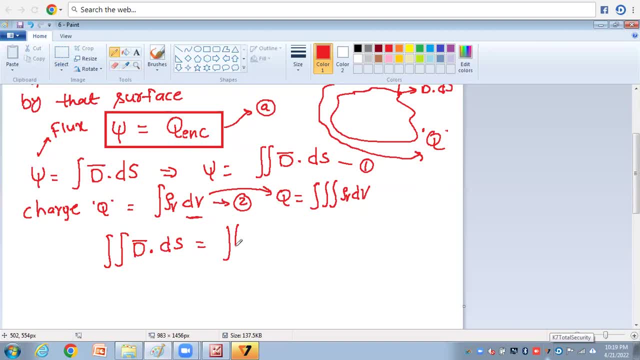 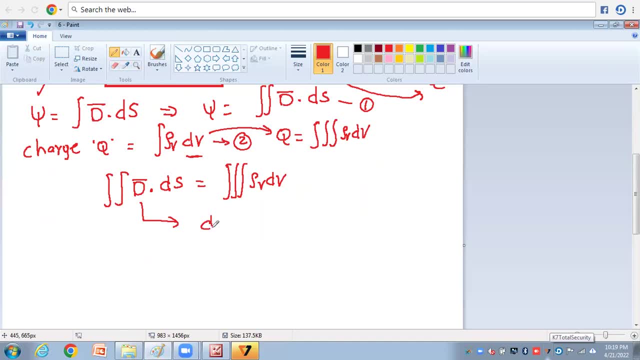 take this expression. we have to apply, we have to apply, we have to apply: divergence theorem now apply. i will write: divergence theorem now apply. i will write: divergence theorem now apply. i will write once again, once again, once again: divergence, divergence, divergence apply, divergence, divergence, divergence, theorem, theorem. 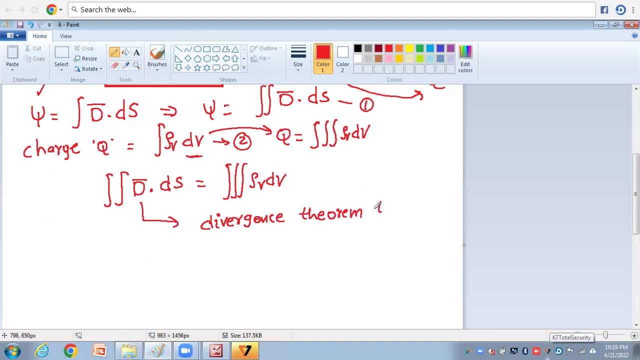 theorem: divergence: divergence: divergence theorem to theorem, to divergence theorem to this term. okay, already we have studied about this this term. okay, already we have studied about this divergence theorem to this term. okay, already we have studied about this divergence theorem. let us take divergence theorem. let us take. 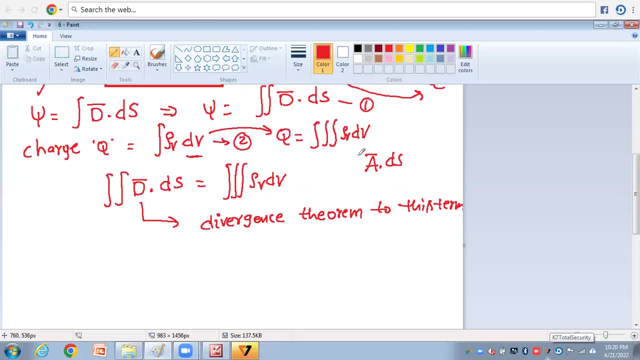 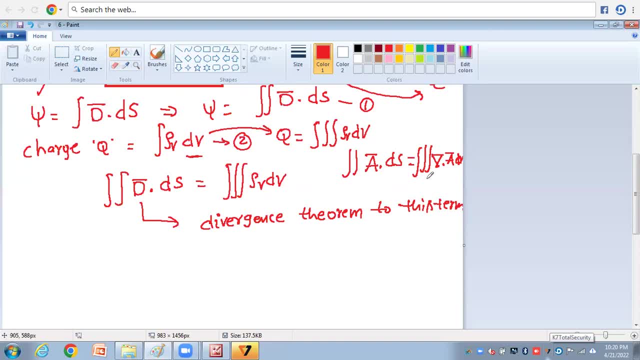 del dot, del dot, a bar, a bar, a bar with respect to db, with respect to db, with respect to db. okay, this is a. okay, this is a okay. this is a about the. about the, about the divergence theorem. again, i will write about divergence theorem. again, i will write about 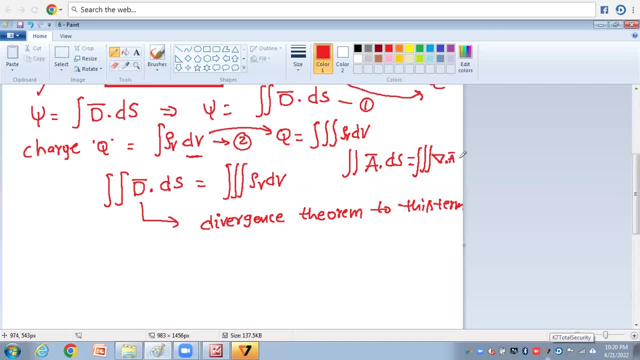 divergence theorem. again, i will write about this divergence theorem, this divergence theorem, this divergence theorem del dot. a bar dot del dot. a bar dot del dot. a bar dot d d d. okay, okay, okay. now, when i applying divergence theorem to: now, when i applying divergence theorem to: 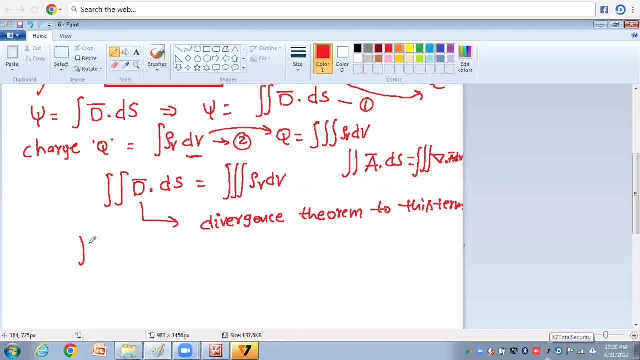 now when i applying divergence theorem to this term. so this is converted to this term. so this is converted to this term. so this is converted to triple integral. so this double integral, triple integral. so this double integral, triple integral. so this double integral d bar dot, d bar dot. 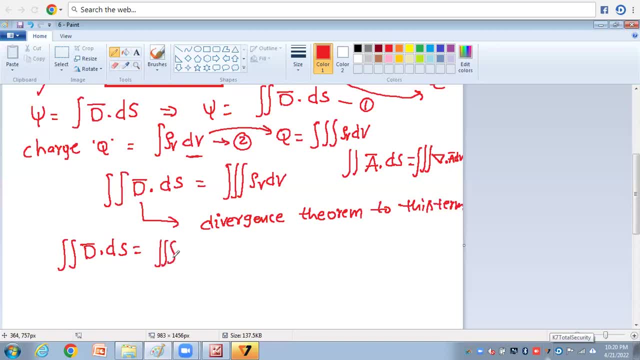 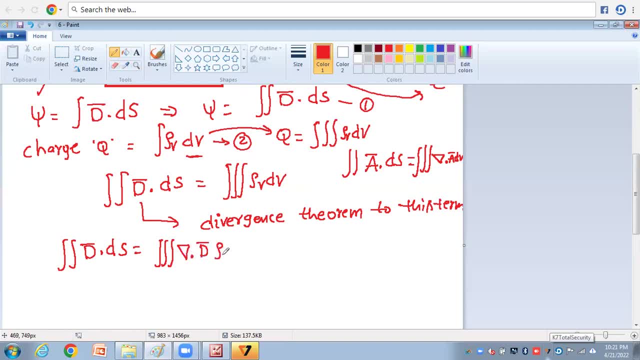 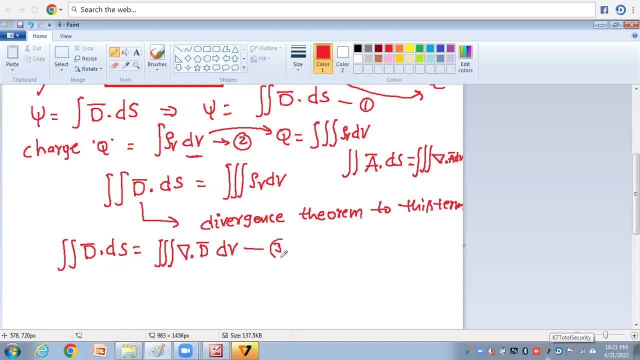 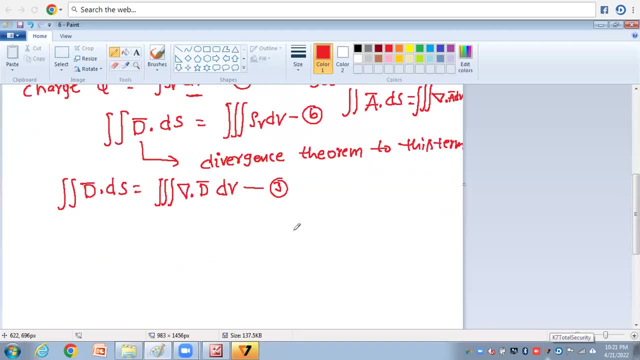 okay, del bar d bar is equal to okay, del bar d bar is equal to. now again, this is expression. now again, this is expression, now again. this is expression: three, three, three, three. substitute in substitute in substitute in expression d expression, d, expression d. okay, now, what happened?